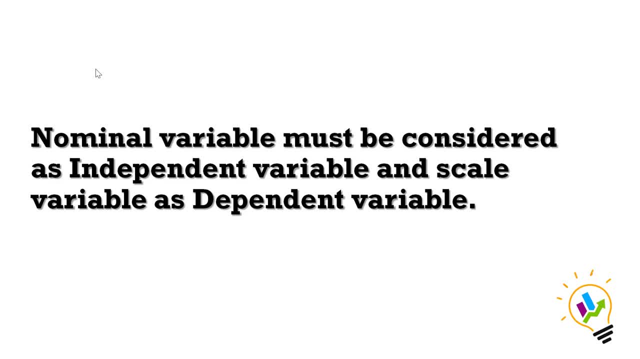 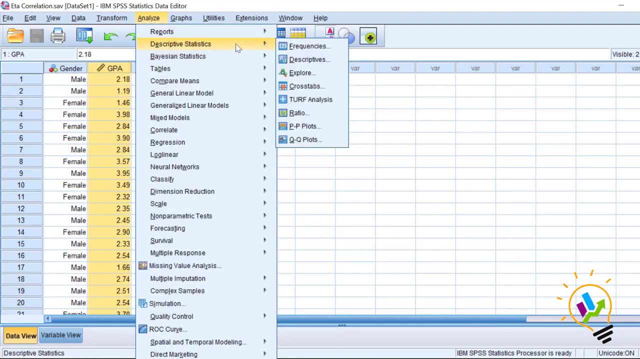 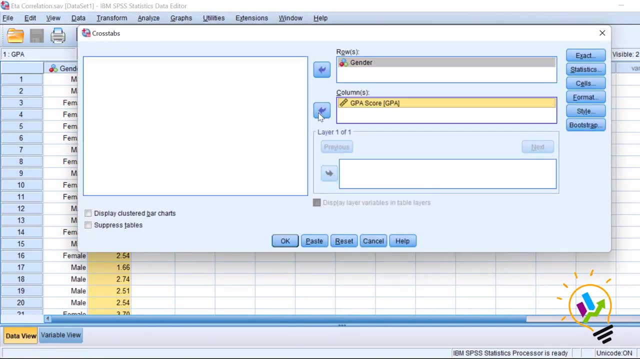 variable are taking out independent variables. Now let us do the analysis In this analysis. first click on analyze descriptive statistics. cross table In this gender as a row and Gps score as a column and click statistics and select this Eta value, because you need to consider the short associatedبر. 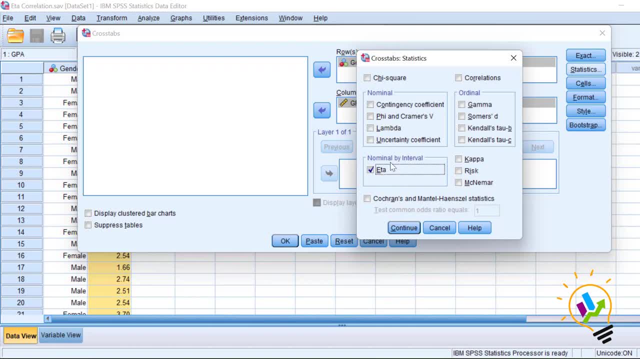 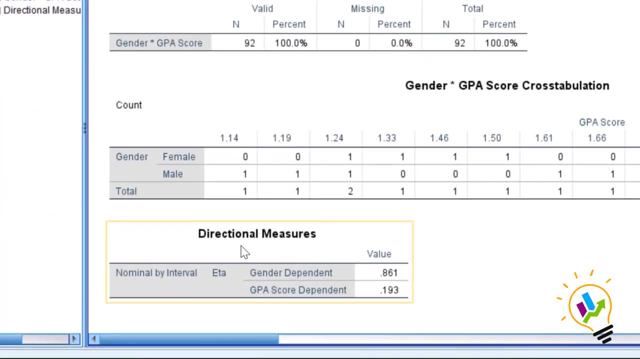 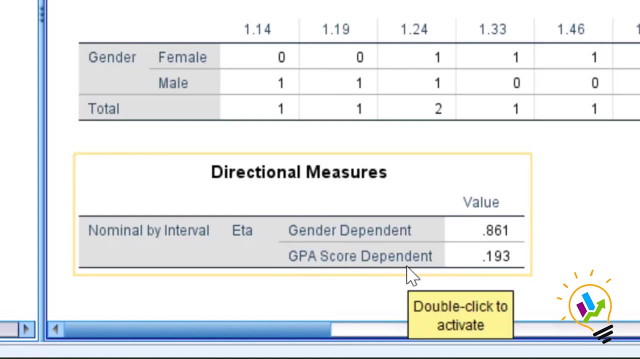 we are going to have a correlation between nominal variable by interval variable, click continue and click ok. now, here you see the directional measures in this. important thing is you must see about gps score, which is a dependent, because, already said, nominal must be independent variable, and the scale 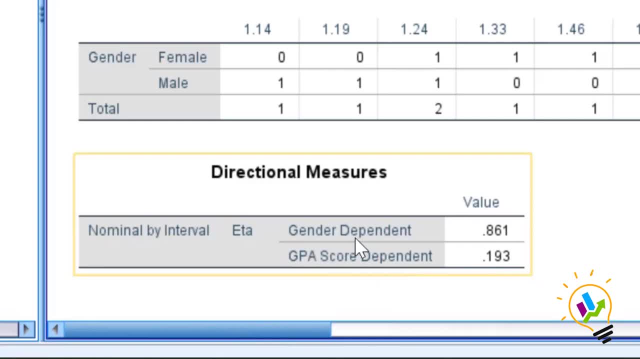 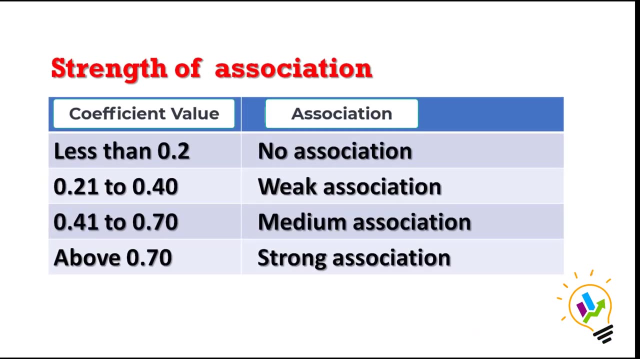 data must be dependent variable. so you must not see gender dependent variable. this variable must not be seen. this value must not be seen. you must see gps score, which is a dependent. here the value is 0.193. now let us see the association of this. so we know that the associate, the coefficient value. 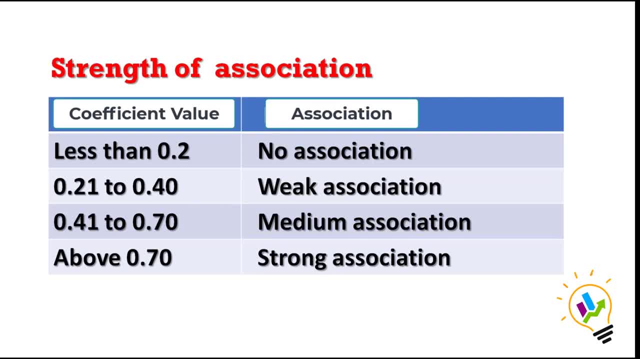 of the correlation is 0.193, and the strength of association: if it is less than 0.2. no association if it is between 0.21 to 0.4. weak association: if it is between 0.41 to 0.70, it is mean. 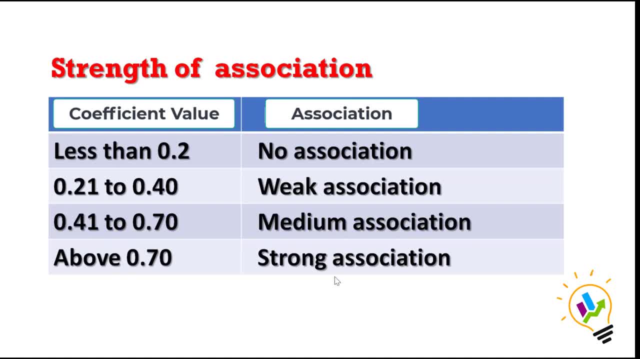 association above 0.7. strong association since in our case we got, the coefficient value is 0.193, which is less than 0.2. so there is no association between gender and gps code. now how to find the significant value for significant value, you must do correlation analysis. 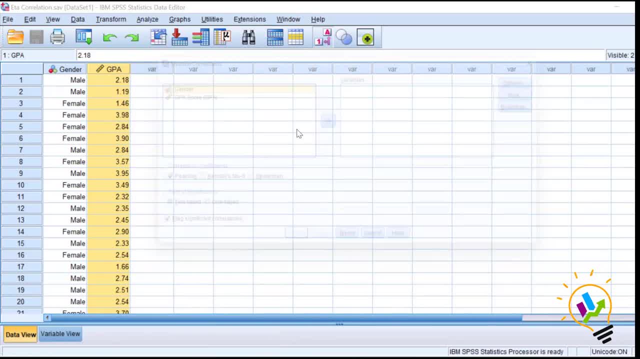 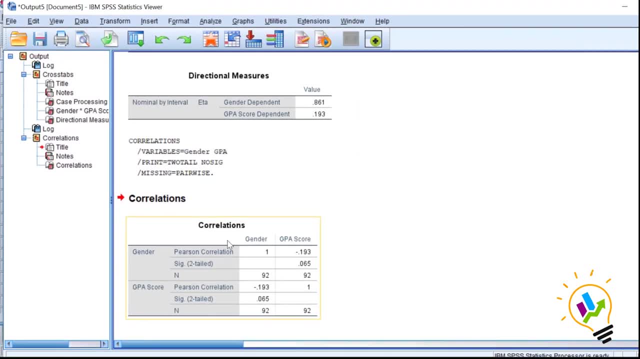 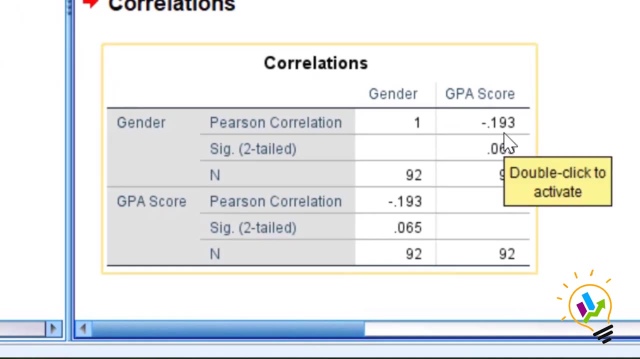 analyze correlation by variant. in this, select the two variables as variables and click ok. now in this correlation you can see the gender to gpa. it is minus 0.193. we already got in eta correlation. the association is 0.193. here we are going to only see the significant value. the significant value: 0.065. if the significant